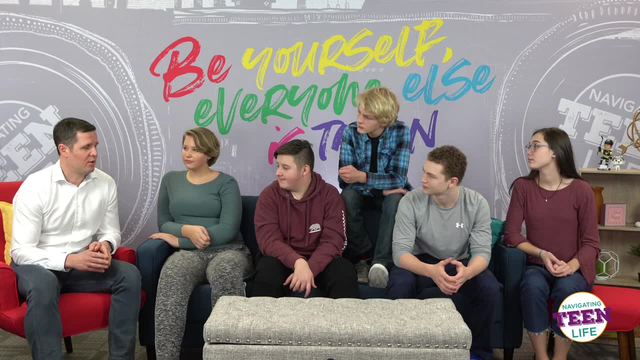 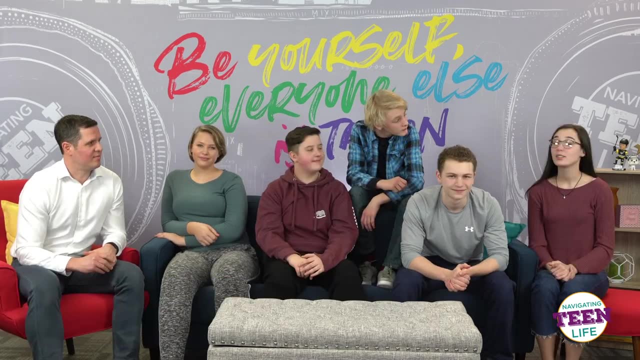 weekly expenses and knowing where your money is going from that point on. There are a lot of tools you can use, either online or just a simple Excel spreadsheet, to help you track your goals. So, Andrew, I'd like to save up for a car. Do you have any tips for me? 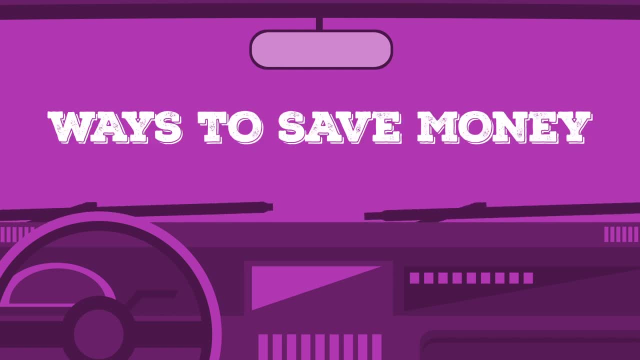 Sure Savings is an important part of financial management. One of the easiest ways to do that is, if you have a job, have your employer make a direct deposit into a savings account for you. Otherwise, you could just take any percentage of your income, whether it's your allowance. 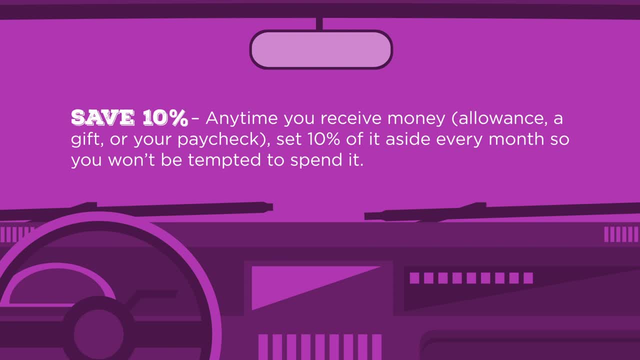 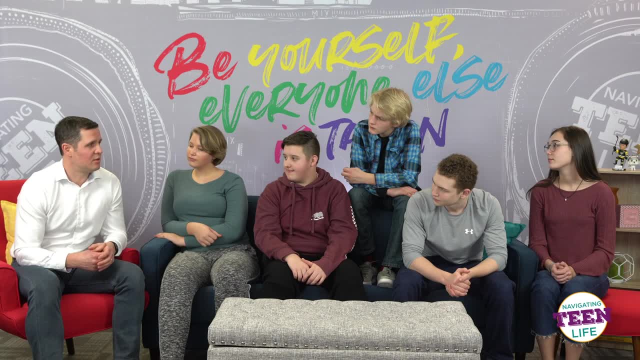 you can save up for a car. you can save up for a car, and if you put it away, it'll prevent you from being tempted to touch that money later on. So you mentioned a savings account. Is that something I could set up? What about like a? 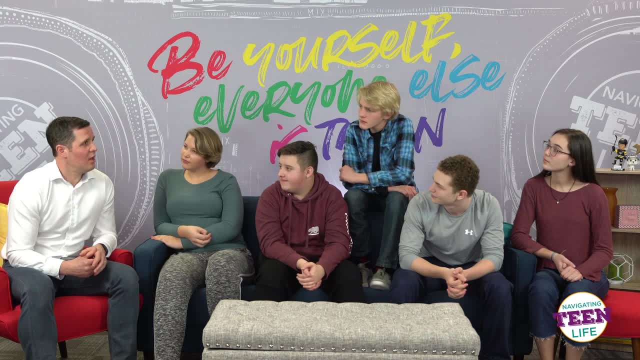 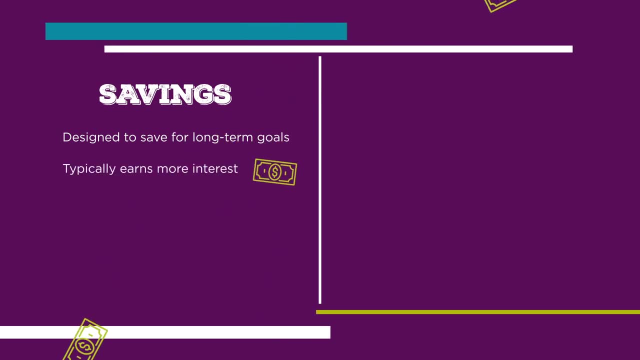 checking account. Sure, That's another great question. Savings accounts. most banks require that you're at least 18 years old. If you're under 18, your parents can go and help you out by opening that account for you and your benefits Once you have that account open. 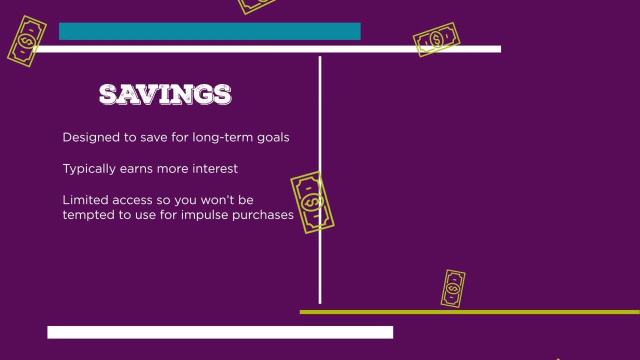 you are able to deposit money in and out of it. The main difference between a checking account and a savings account is: with a checking account, you're able to write checks and use a debit card that allows you to make payments elsewhere. A savings account is more of a longer term place to park. 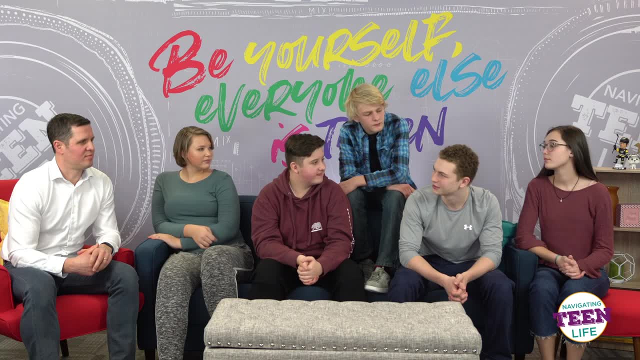 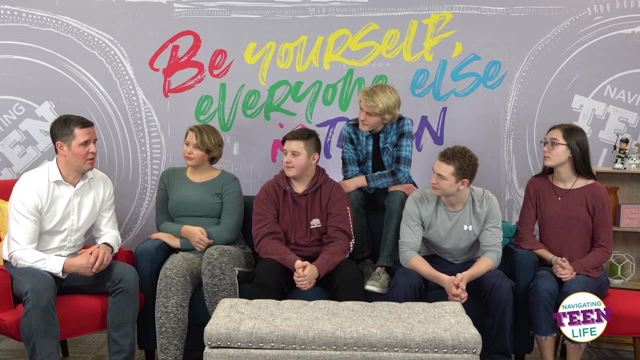 your money. I'm a junior and I will be heading off to college soon. Should I be needing a credit card? That's a great question. Credit cards are a necessity for modern day life anymore, with online shopping and just the ease of not having to carry cash around. But there are. several dangers associated with opening a credit card. First off, with modern laws, you need to be at least 21 years old to open that card, or 18 and have a co-signer. The dangers of credit cards is when you overspend and use your credit. 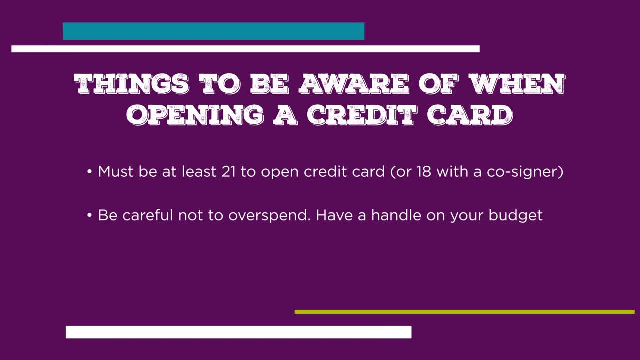 card to buy things that are unnecessary. It's important to have a handle on your budget first, like we talked about previously, before opening a credit card, because high interest rates can make repaying that debt very difficult. So we spent a lot of time talking about savings.